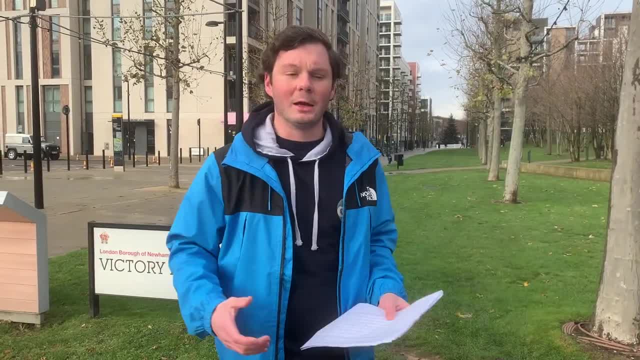 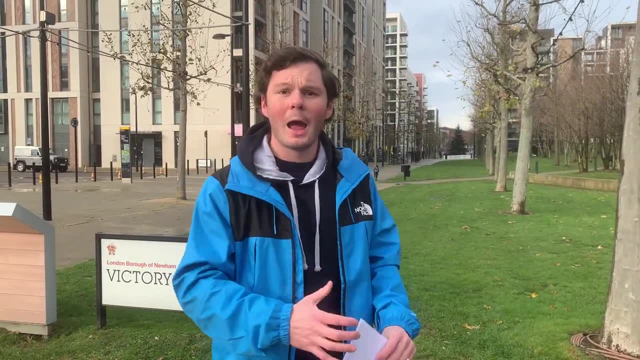 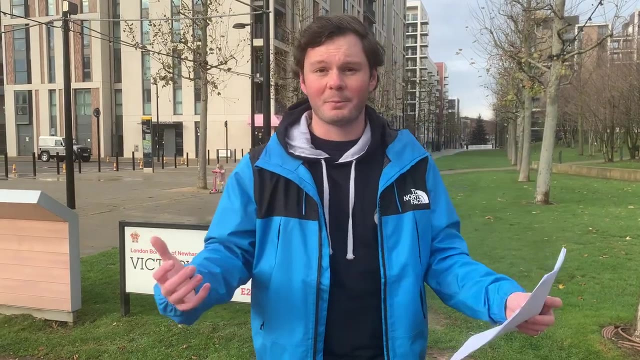 consider is: how has this area changed from about half a kilometre away in Stratford-Newtown, which was very much a residential area. I want to consider how has the environmental quality changed? If we look around here, can you see much litter, can you see many trees, much green space. 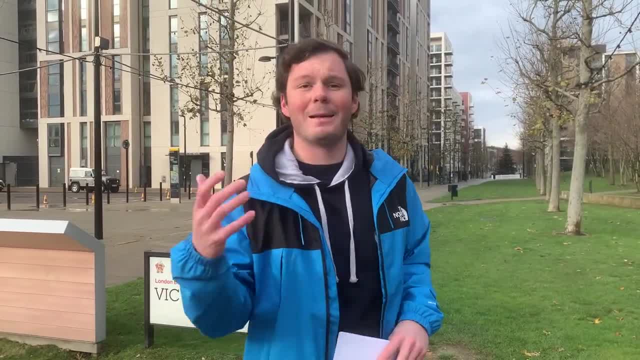 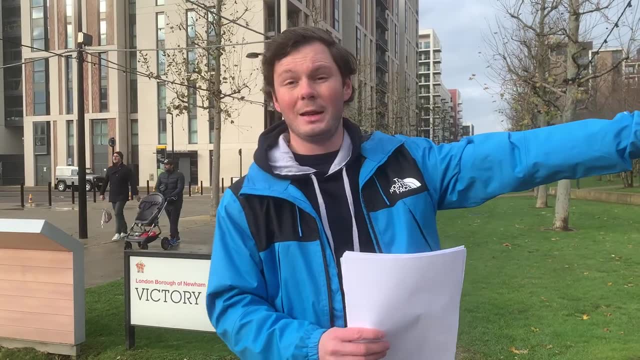 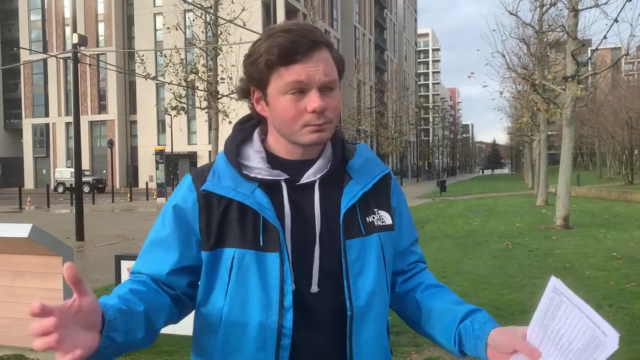 can you see homes boarded up? can you see abandoned buildings? I want you to consider all these things, to see how has regeneration now changed, from only half a kilometre away, in Stratford-Newtown, to now here at the Olympic Village, here in East Village. So to be able to 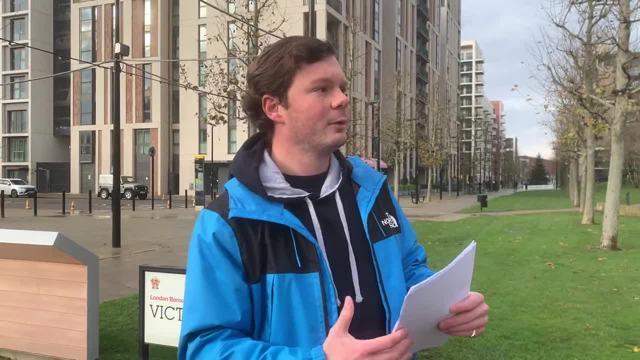 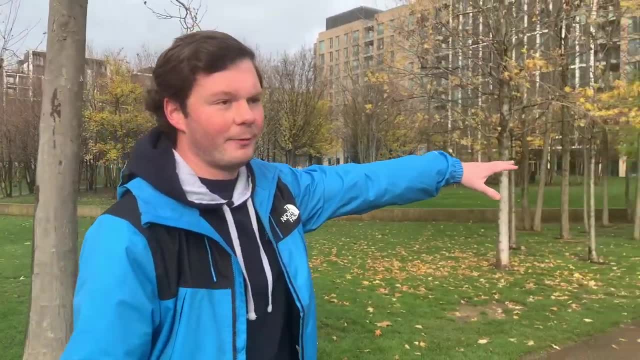 start to consider these things. we're going to continue collecting data. So what we're going to do is continue with our systematic, stratified and random samples, where we're going to start off about 50 metres away here, So doing this as a systematic sample, every 50 metres we'll collect. 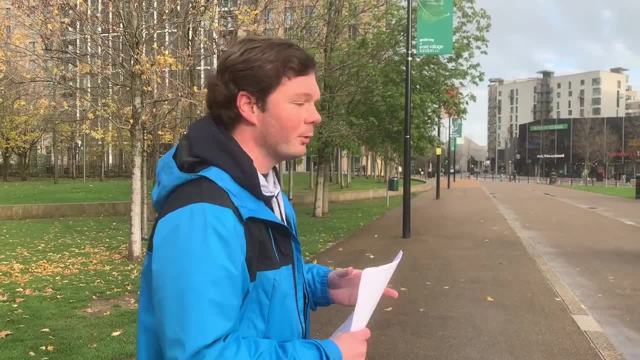 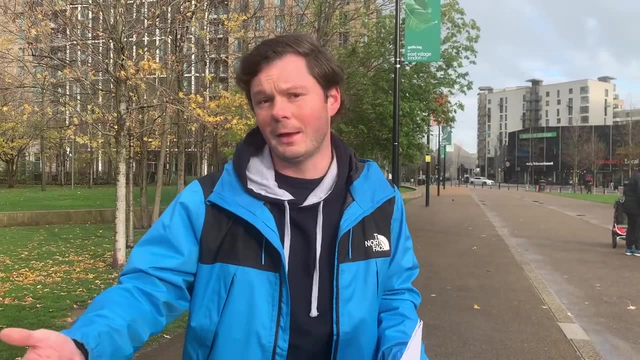 data and we're going to do 50 metres just before the Sainsbury's local. there You're going to do your traffic counts. you're going to do your traffic counts. you're going to do your traffic counts- people counts. you're going to do your environmental quality survey. you're going to do all of these. 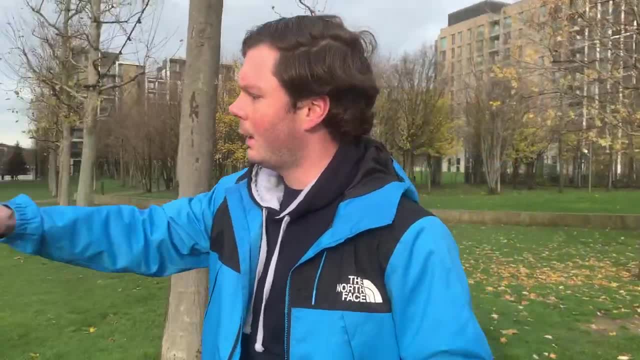 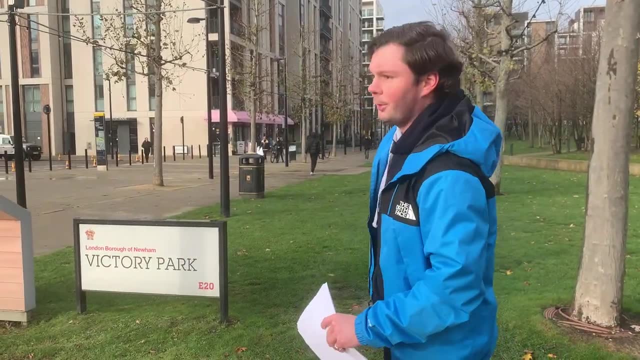 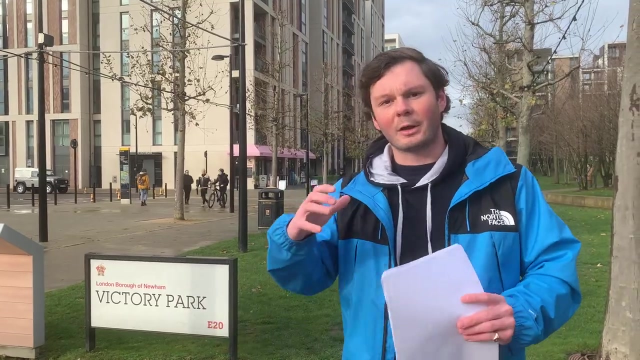 things and then, once we move on, we're going to move on to here, 50 metres away by Victory Park, sign here, and that's where we're going to do our next data collection set. And, once again, our third site is going to be 50 metres down there, so that we've now got a consistent method to be able to. 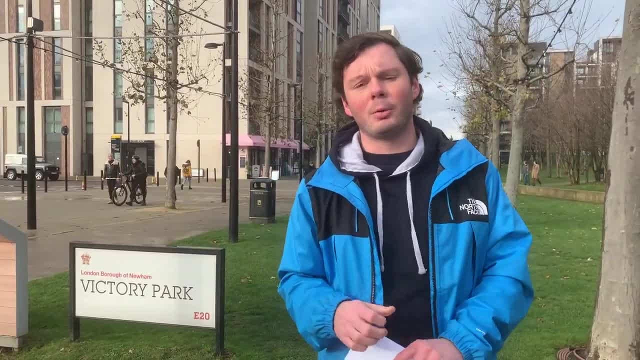 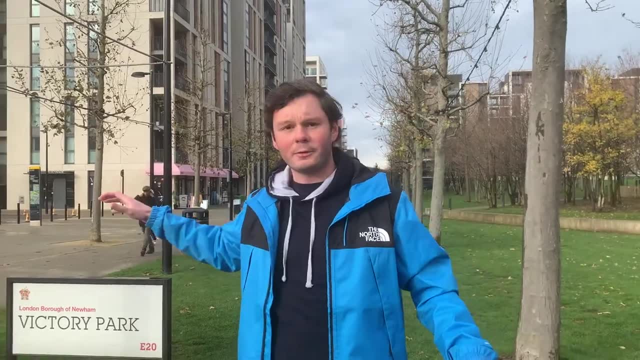 collect data all the way through. There is, however, a problem when we're doing this, When you're doing a systematic sample of, say, every 50 metres. that is great, so that we've now got three sites, but what about if you miss something that is within? 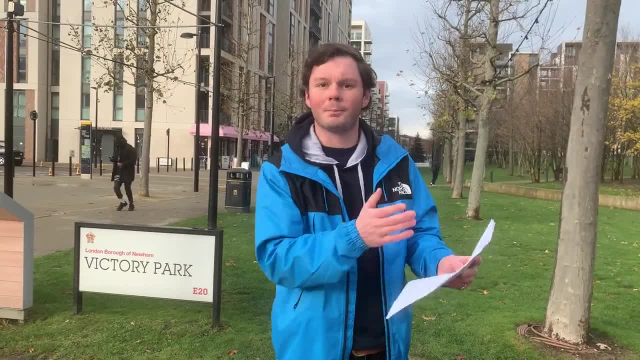 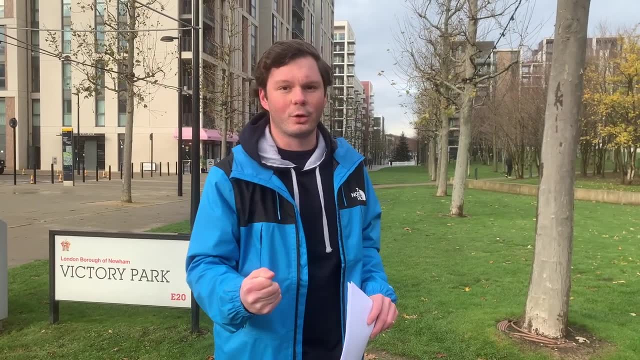 the 50 metres. What if there's some data that you weren't able to collect because you did it every 50 metres? That's something you must consider and think about: how reliable is the data you're collecting? How accurate is this data collection method? But there's one other thing that I want. 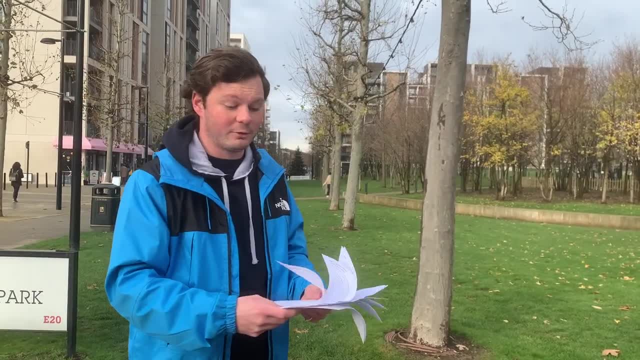 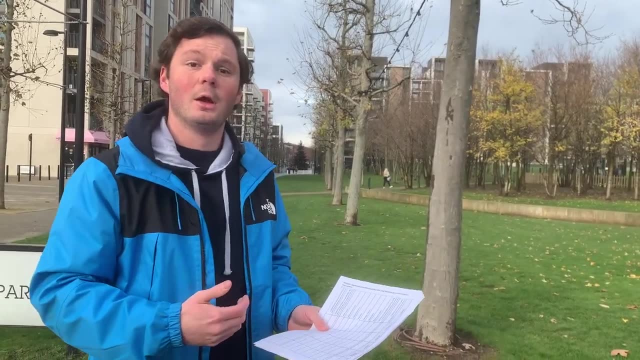 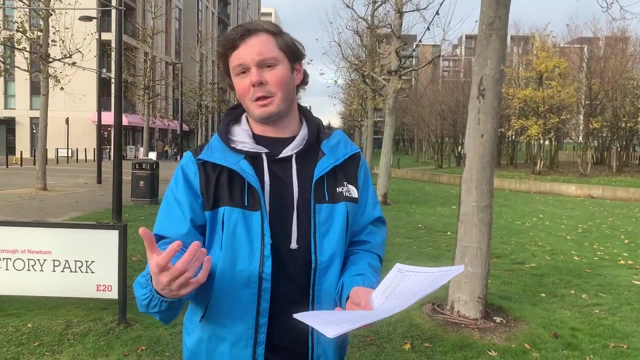 us to consider when we are doing this: data presentation, data collection. sorry, and that is an interview. We will do questionnaires at our three chosen sites, So you'll do this at three different points at our three chosen sites. Now, a questionnaire being a qualitative data collection method is a really interesting way.